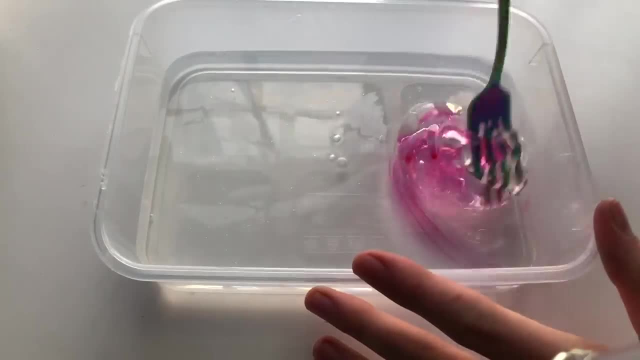 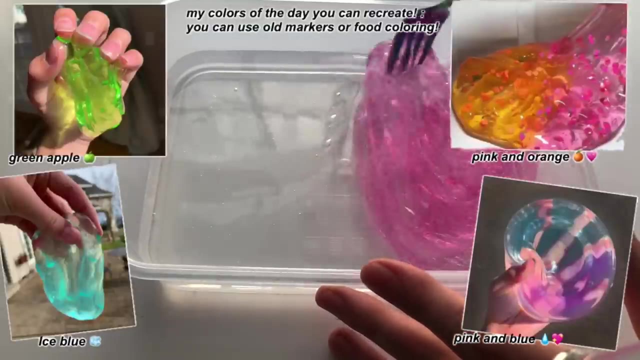 it is time to have the fun part, which is coloring the slime and making your slime however you want it to look. If you have a clear shampoo, you can do a lot of different colors and stuff using markers or food coloring, but if you don't have a clear shampoo, you can do a lot of different things also. 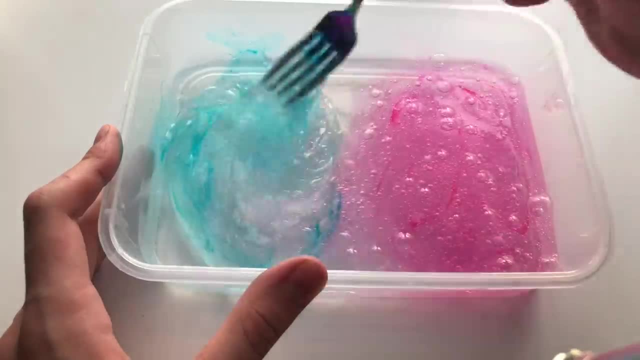 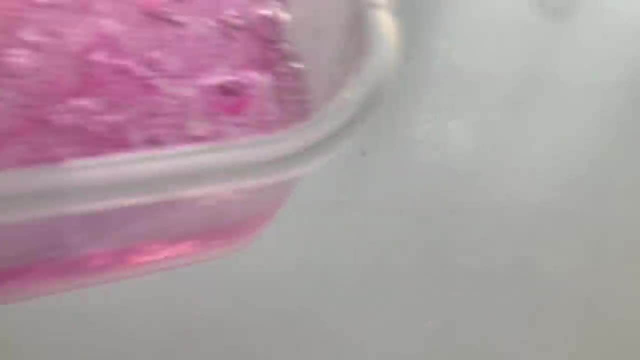 I transformed my slime to be pink and blue, and I think it looks really cool. Now is when you will be needing water, so you just want to put a thin layer of water on top of the shampoo without mixing it, and now we're going to put this in the 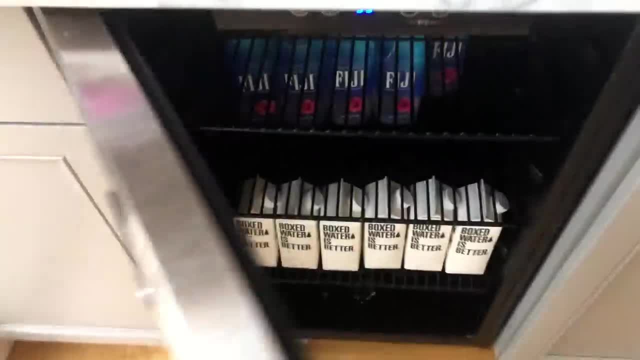 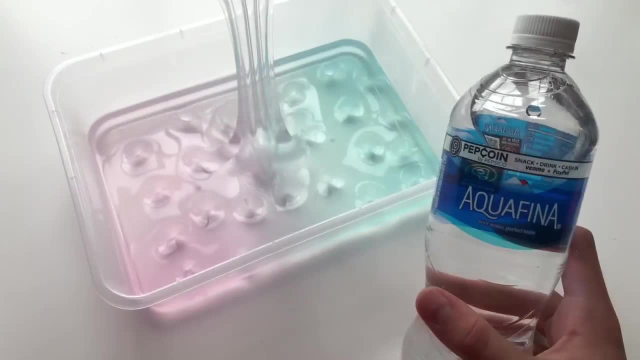 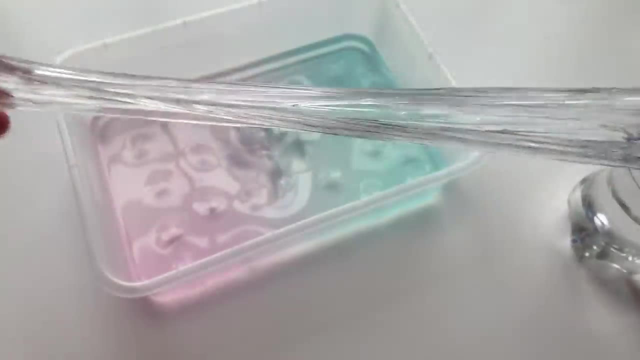 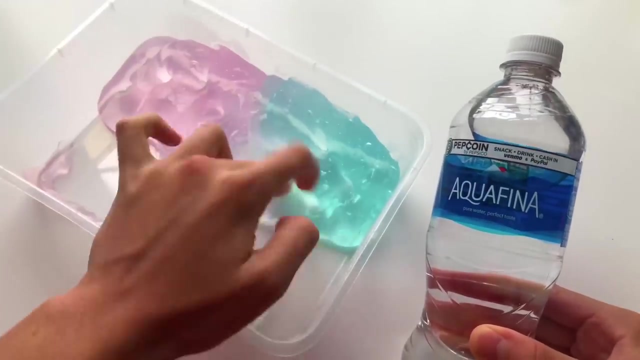 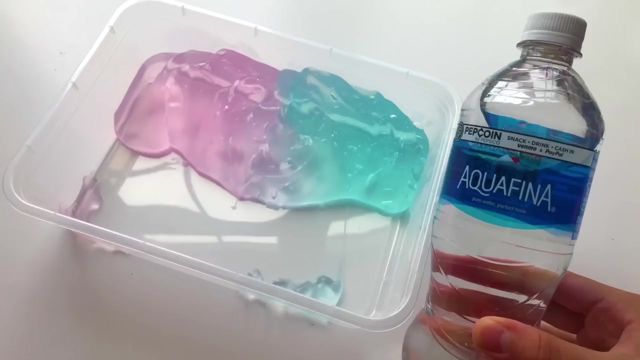 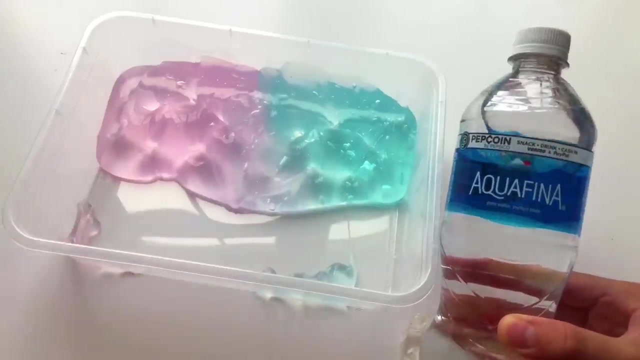 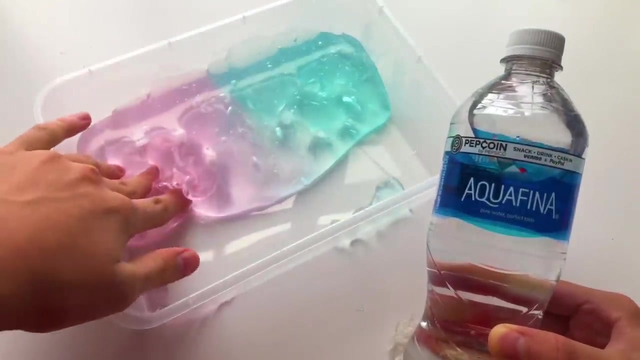 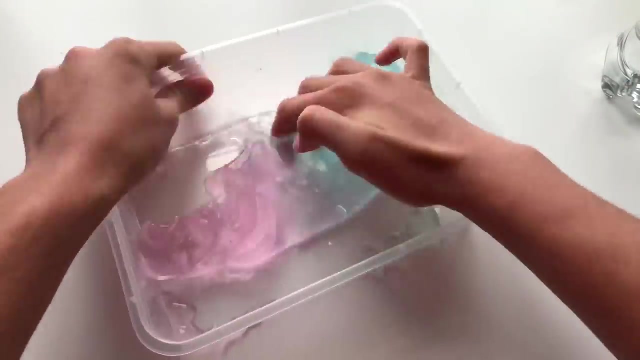 refrigerator. We are going to put this away in the fridge, put it in, and our slime will be done. when we take it out, I'm going to show you guys how water slime looks. So let's do this. just like slime, but it's made out of ingredients you already have at home and 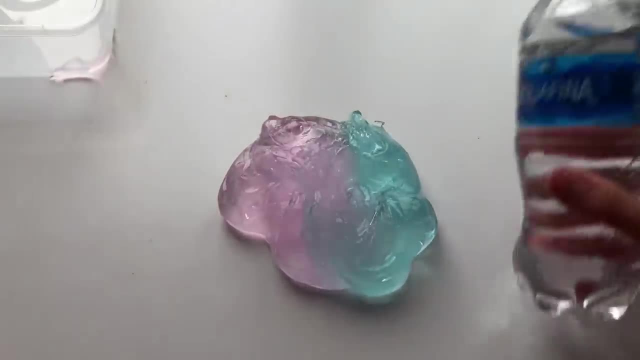 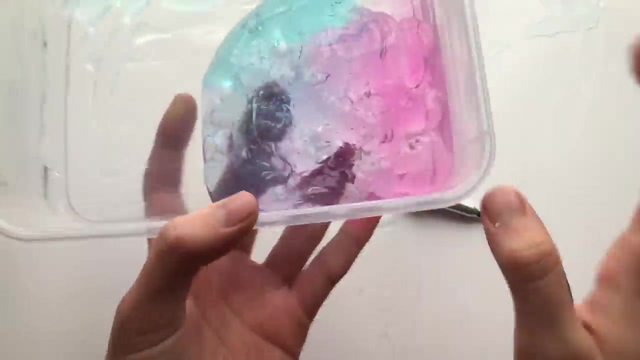 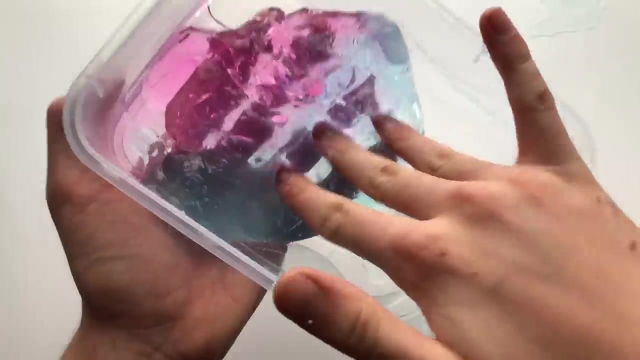 it's really, really fun to play with and it looks really cool. this water slime is currently one of my favorite shampoo water slimes. I really love water slime and I've been playing with this one for about a week now and I'm still enjoying it a lot. I know you guys are not gonna want to miss the next recipe because we 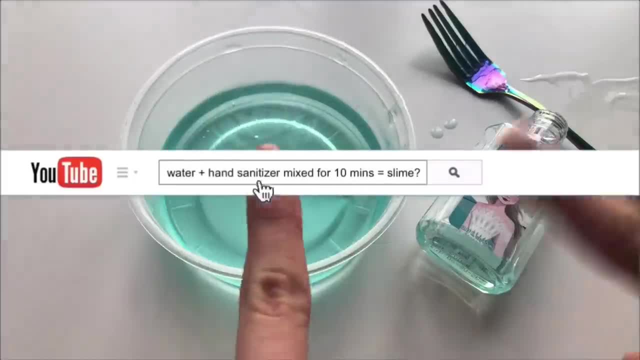 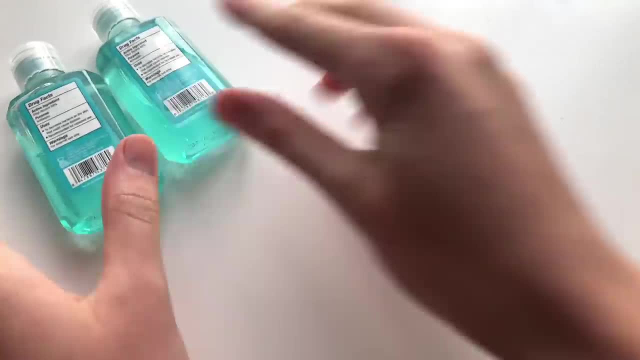 are about to test out the hand sanitizer water slime because I feel like we're all using hand sanitizer so much, especially recently. I thought I would test out an interesting hand sanitizer water slime recipe that you guys commented on my last video. but the comments with this recipe that you guys 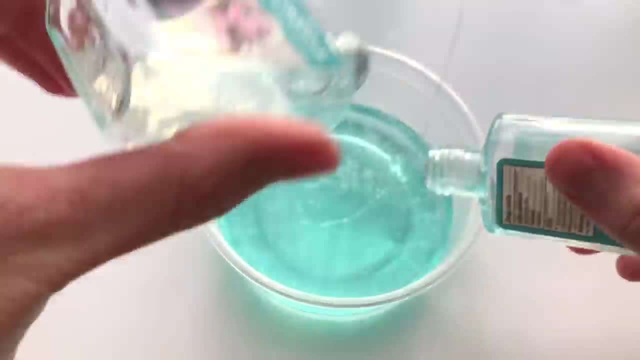 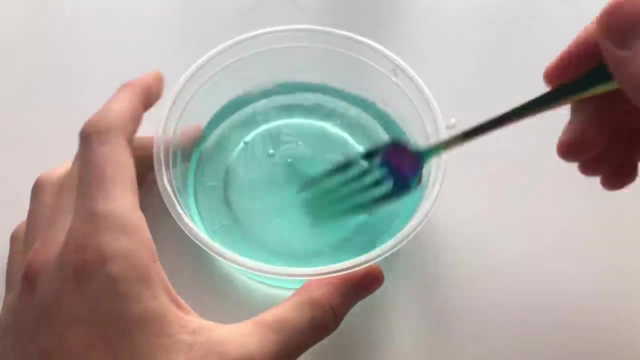 left said that if you take a fork and you put it under the faucet and get it wet and you mix the hand sanitizer for five to ten minutes really fast, it's supposed to make like a little bubbles or something. and you guys said you saw this on a Troom Troom. so we will see if this works. if you didn't know this, 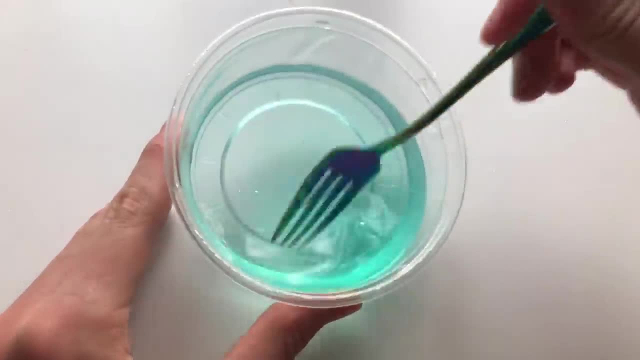 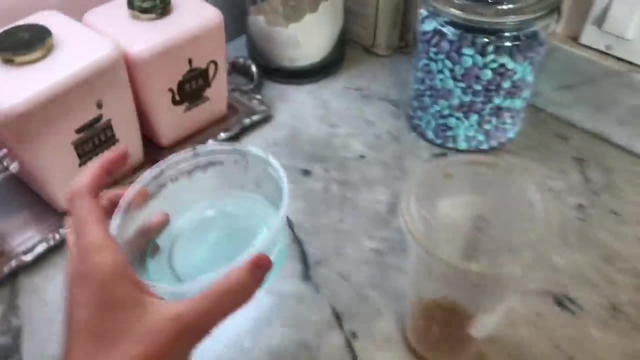 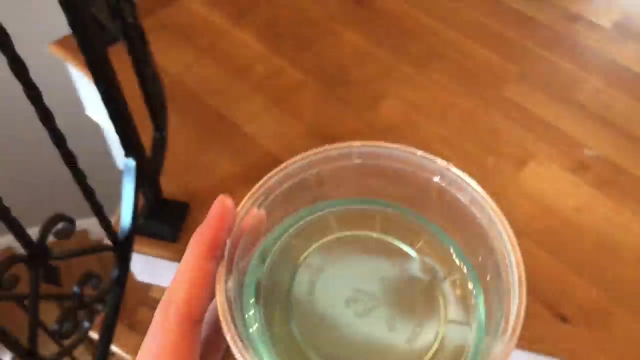 already. hand sanitizer cannot freeze because there's alcohol in it. the water fork hack is supposed to allow it to make things slime. now all we have left to do before we can see if this worked or not is put this into the freezer. it has been about 15 minutes since I put this in the 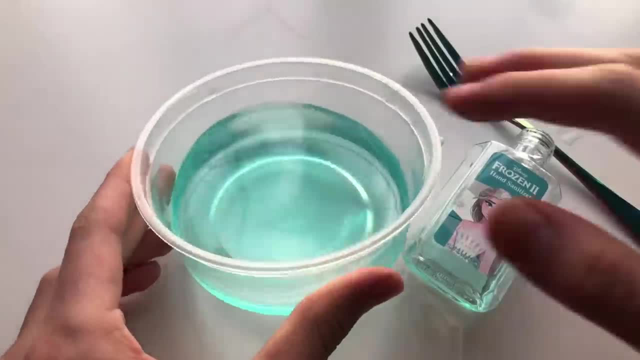 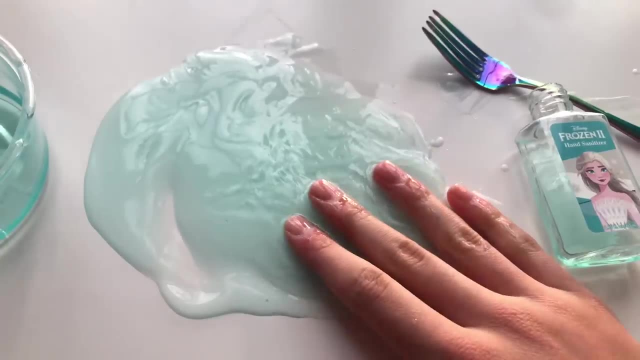 freezer, so we are gonna see if it worked. as you guys can see, this did not work out, which is sad because I feel like it would be cool to be able to make slime out of hand sanitizer. let me know if you guys know any other recipes like this one that I can test and next week to see. 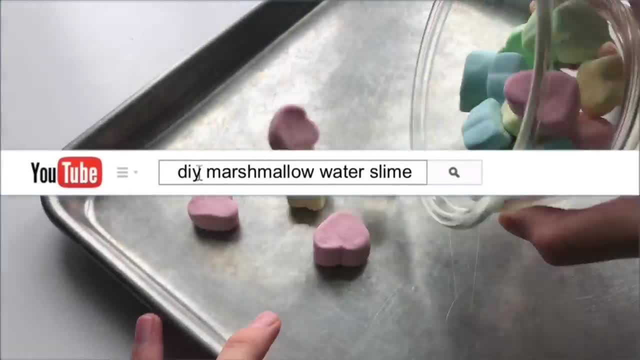 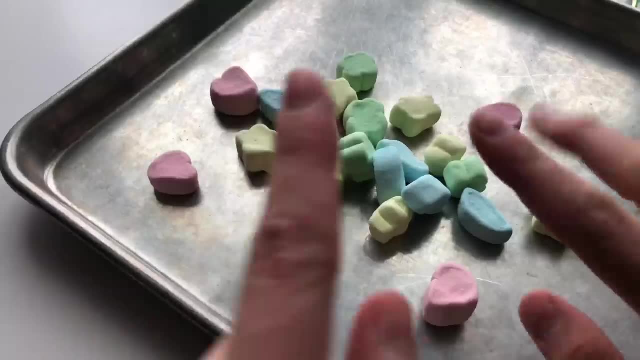 if we can get those to work. slime recipe we are gonna be testing out isn't the marshmallow one, so I'm so excited for this. I got these Lucky Charms marshmallows that are all rainbow colors and I think they look really cool, so I'm gonna just be rearranging them. 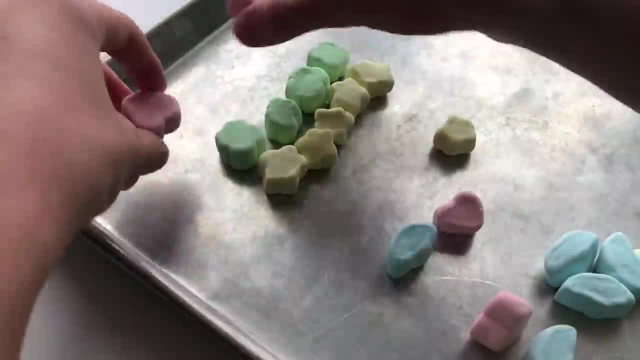 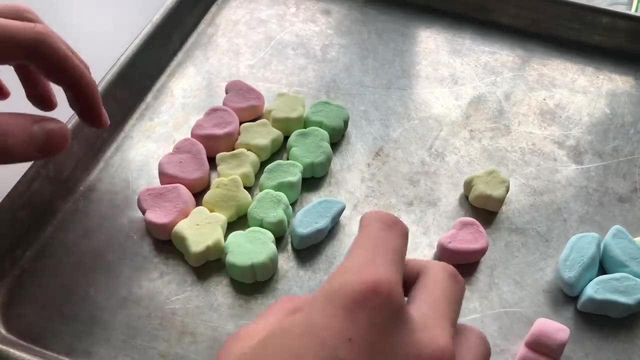 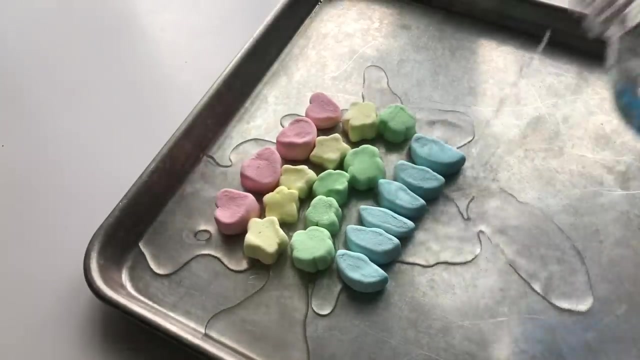 first, I'm super excited to see if this works because it seems like a really fun experiment. and I'm really excited to see if this works because it seems like a really fun experiment. I'm super excited to see if this works because it seems like a really fun experiment. because we are gonna be putting this in the oven and it actually kind of seems like this would make sense, that it would make slime. so we had to put the marshmallows in at 350 degrees for 15 minutes, and here's how the marshmallows: 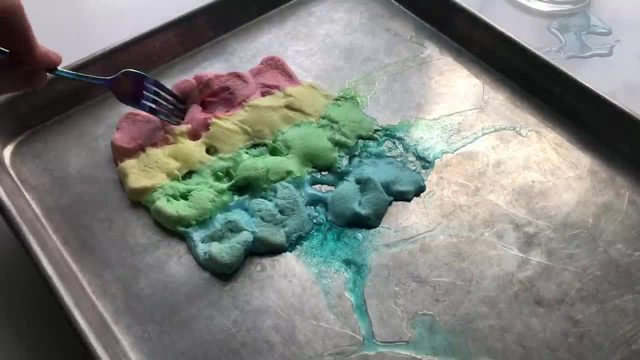 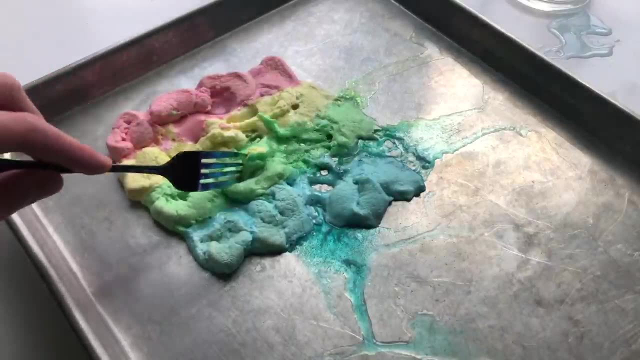 look, they actually puffed up a lot and they just melted together. but we're supposed to let them sit for five to ten minutes until they've cooled down before we mix them around to see if they feel like slime. we're gonna let them sit for five to ten minutes until they've cooled down before we mix them around to see if they feel like slime. 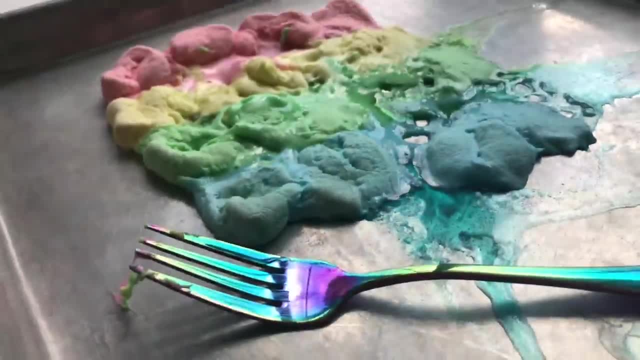 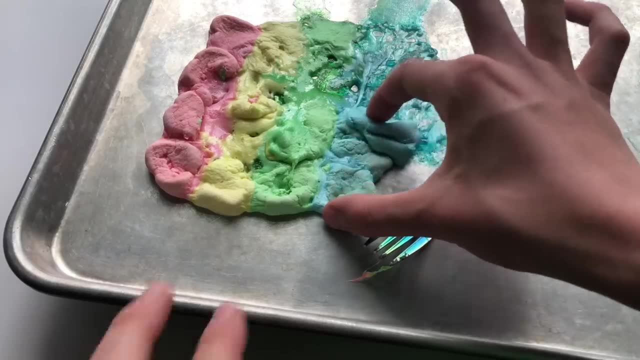 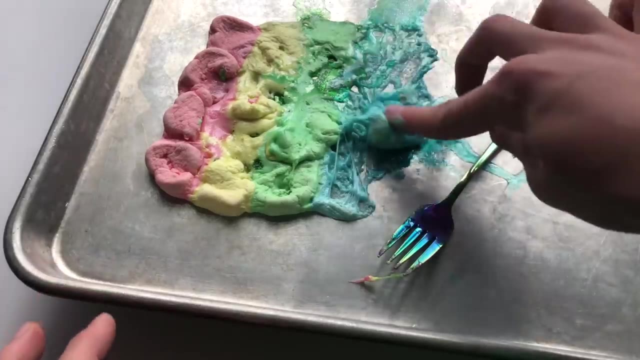 we're gonna let them sit for five to ten minutes until they've cooled down. before we mix them around to see if they feel like slime. let's check the blue one first. so let's see if this one feels like slime. okay, so let's check the blue one first. so let's see if this one feels like slime. okay, so. 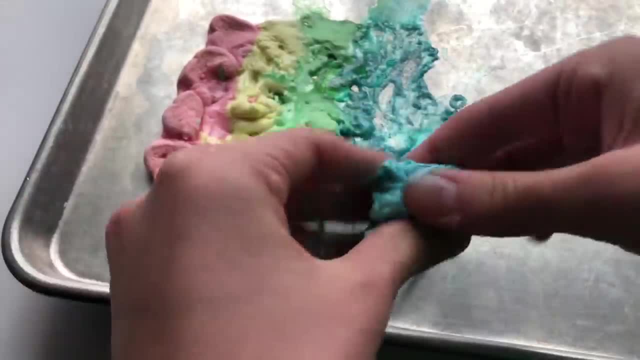 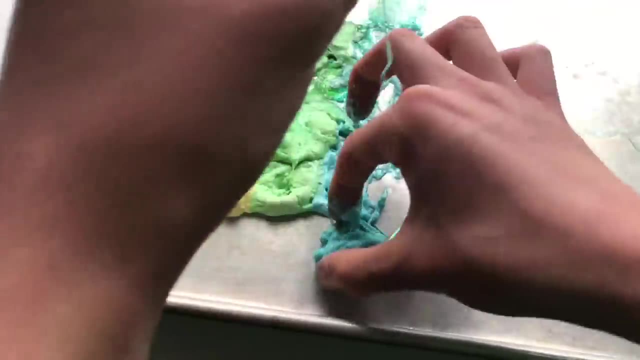 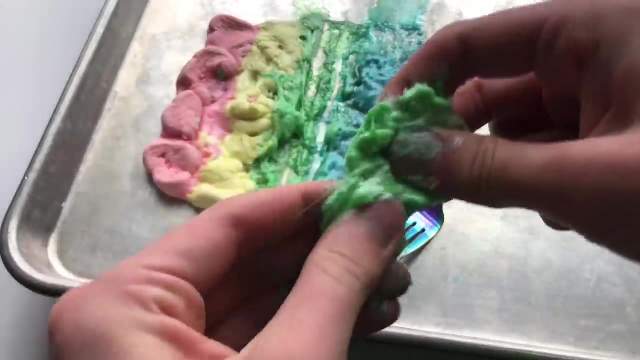 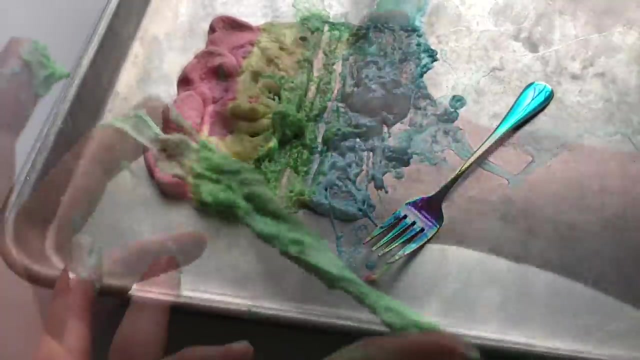 this one feels very sticky, but when I mix it together it's starting to feel a little bit more like slime. it definitely turns into slime when you mix it more and more. I'm noticing that a hundred percent all of these could turn into slime if I just mixed them for. 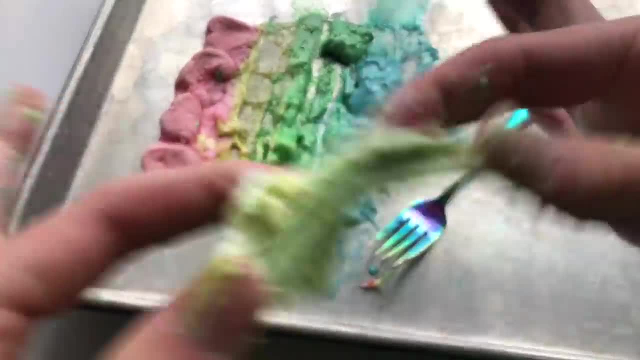 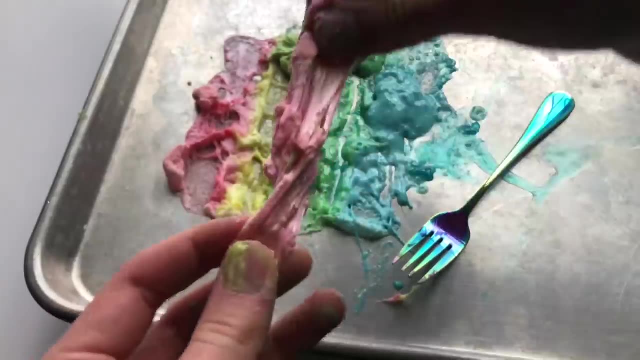 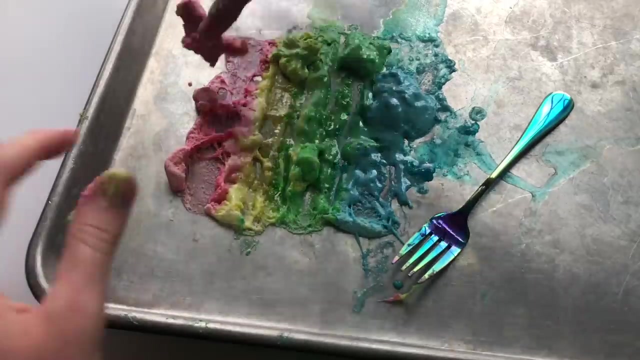 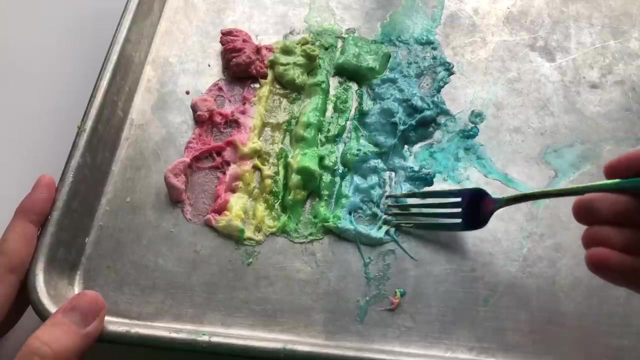 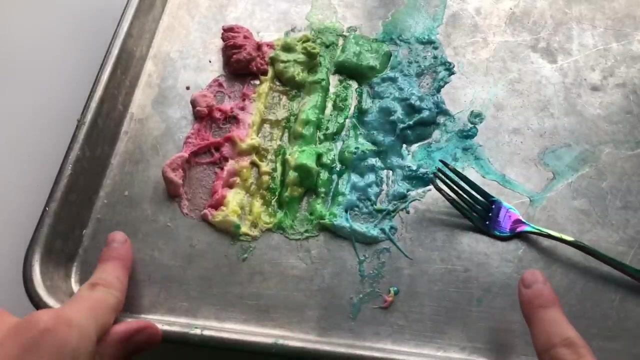 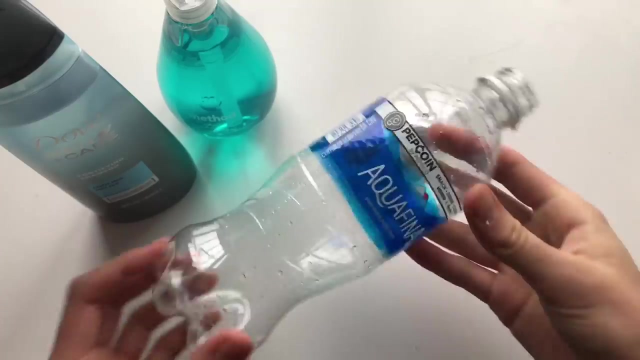 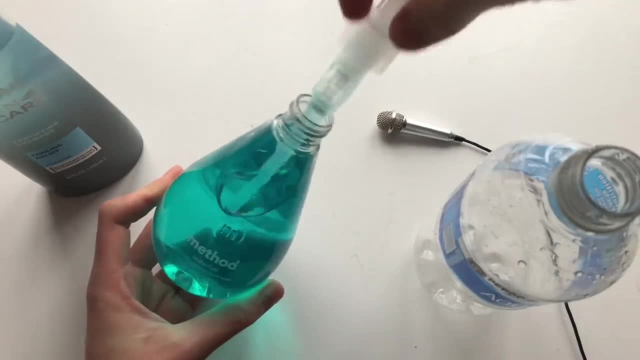 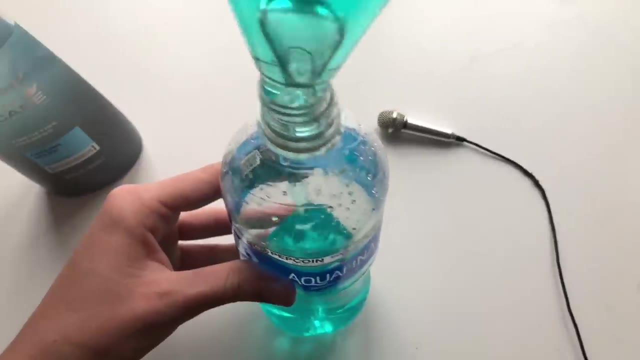 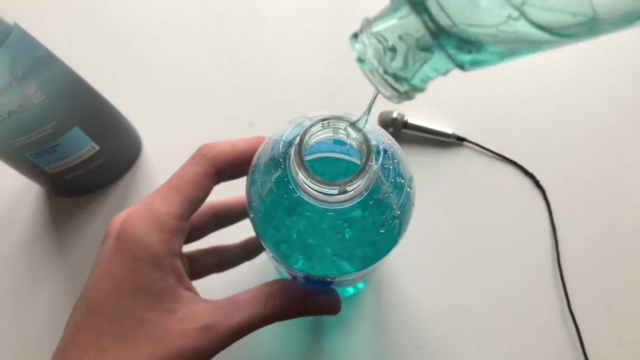 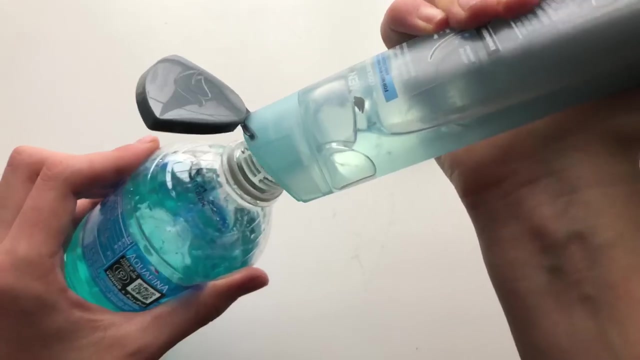 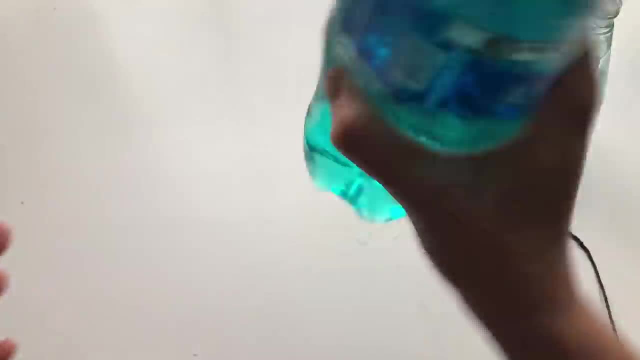 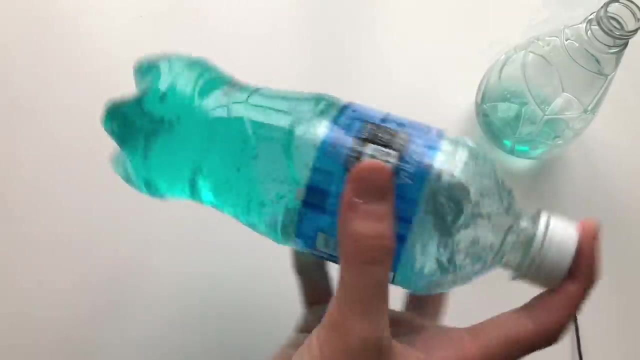 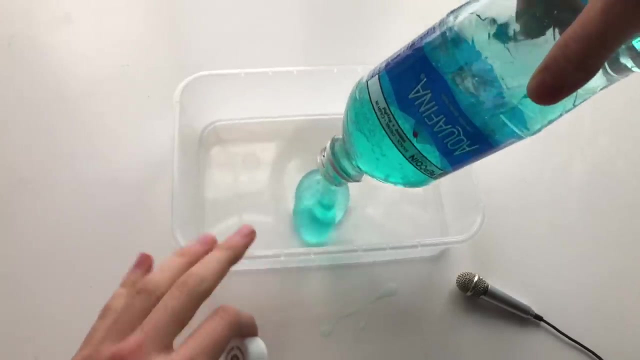 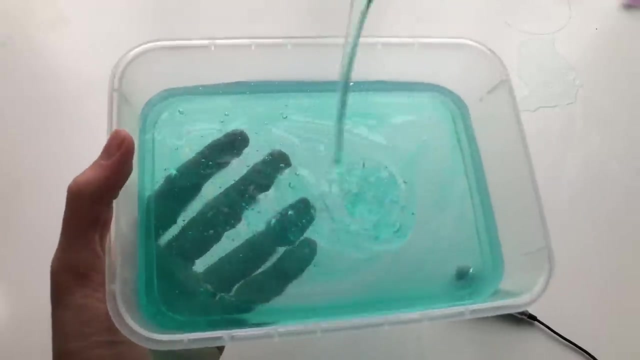 and then you want to mix the two together by shaking it to turn it into a slime. after getting so many requests to make this, I tried it and it worked super well. so this is that recipe and, lastly, all I did is I just poured this into a container that I could put in my fridge. I did have to put this in my refrigerator to congeal for about ten minutes, but here is how it. 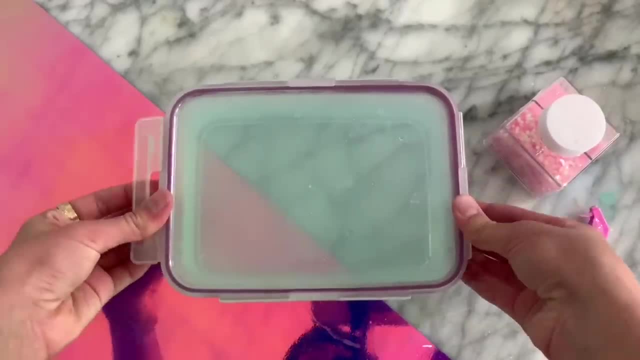 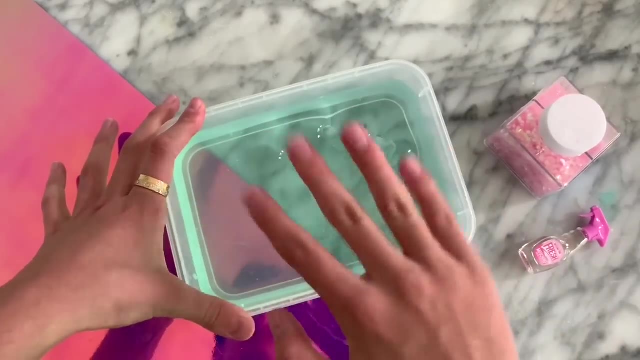 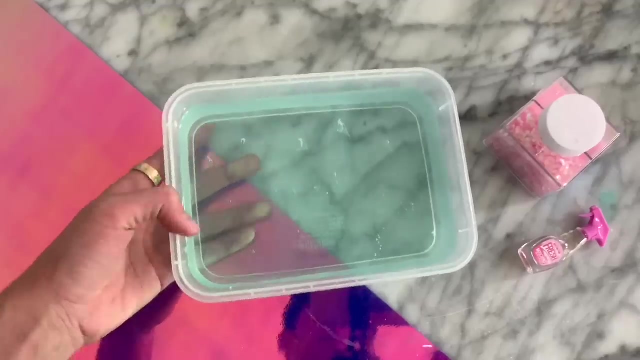 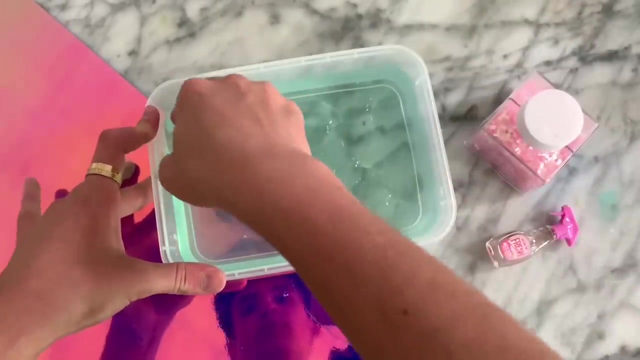 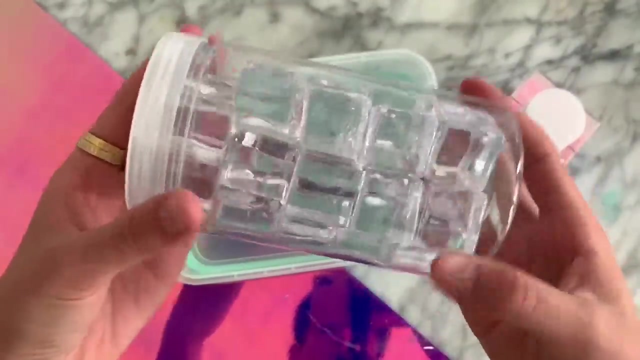 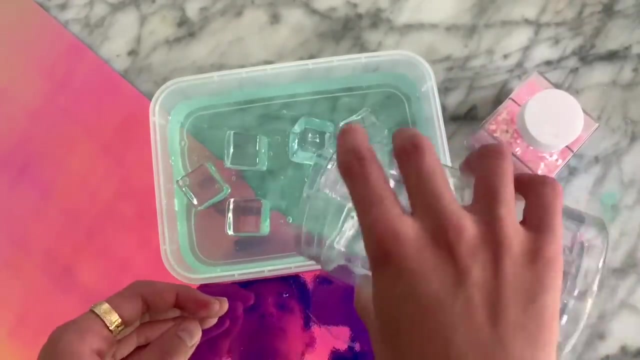 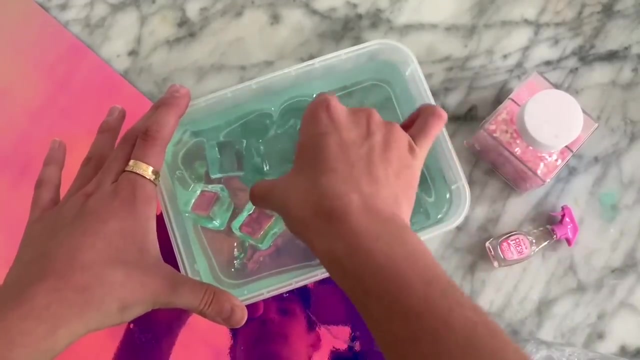 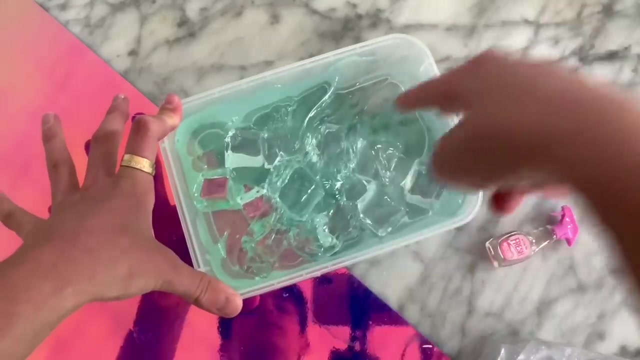 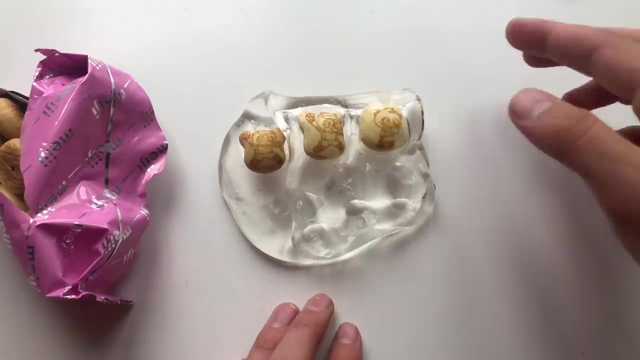 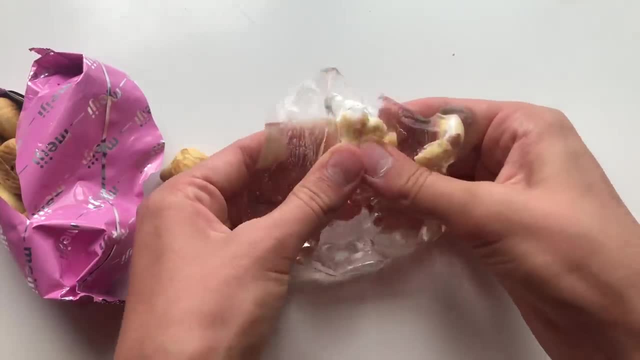 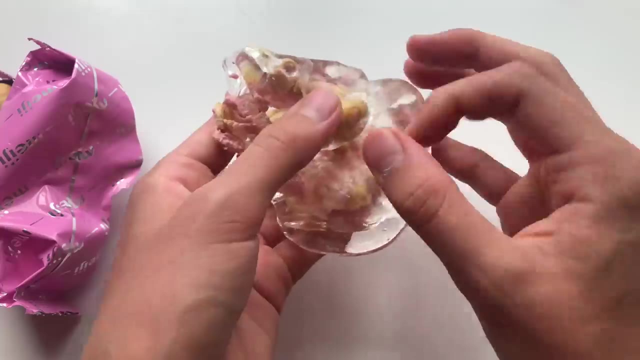 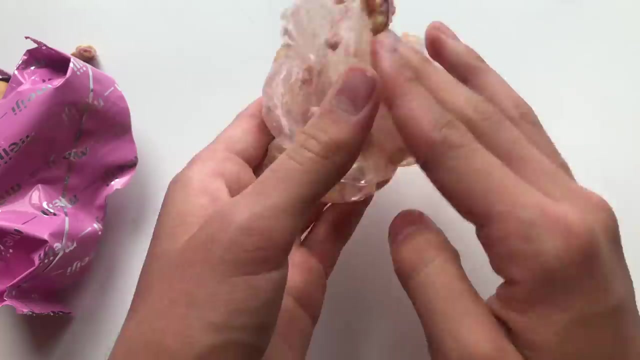 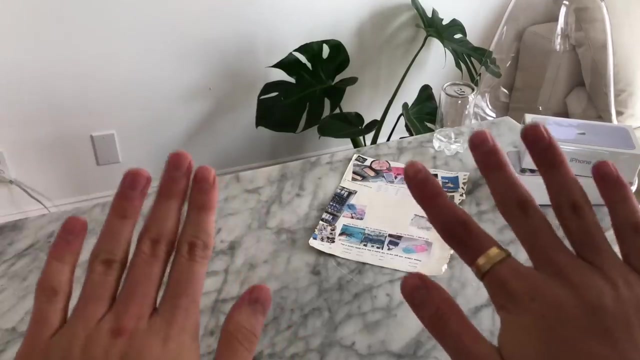 into this clear slime, so enjoy. Cookies made a really cool sound when I mixed them in, but this wasn't the best slime after I mixed everything. I've been really sad recently because it's been a while since I've been able to do a video. 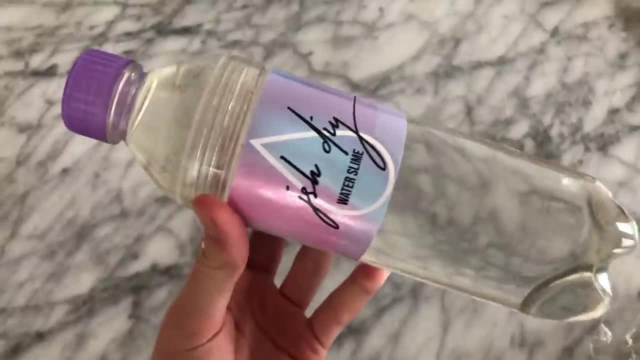 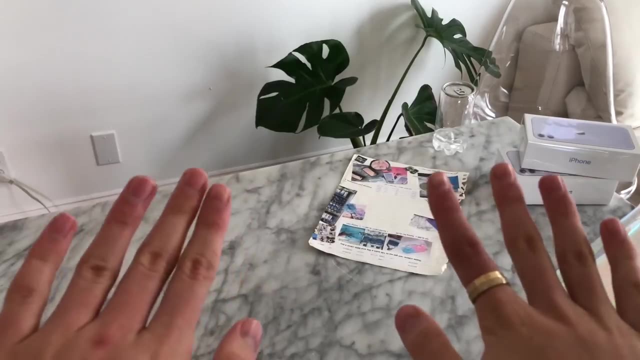 so I thought I would answer a couple of your questions, because I'm back, My bottles are out and I have a lot to talk about, so I got a coffee and I asked you guys for questions, so I'm going to be answering all the questions you guys have. 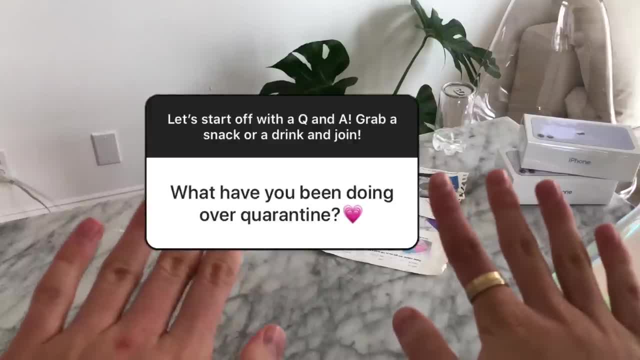 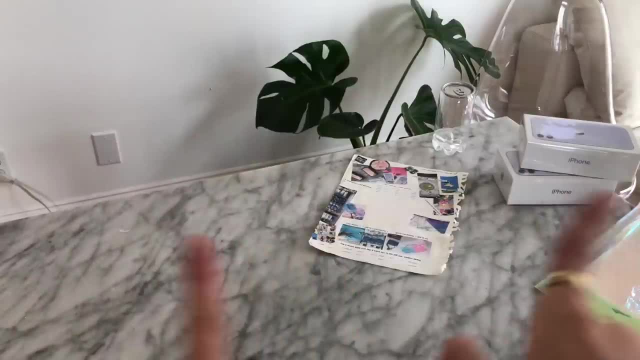 One of you guys is asking where I have been and what I've been doing over quarantine. so I've been pretty busy with school and that's why it's been a bit since I've gotten to talk to you guys. but I've been really busy with school and I also redid my studio. 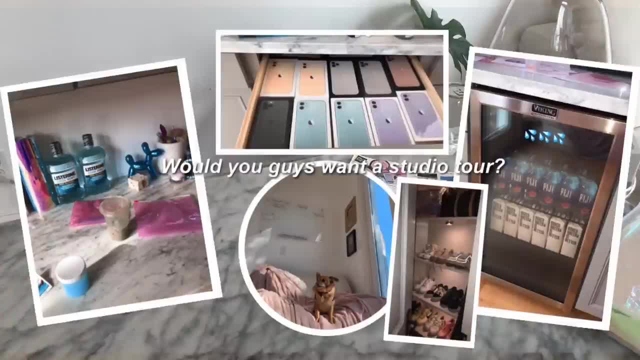 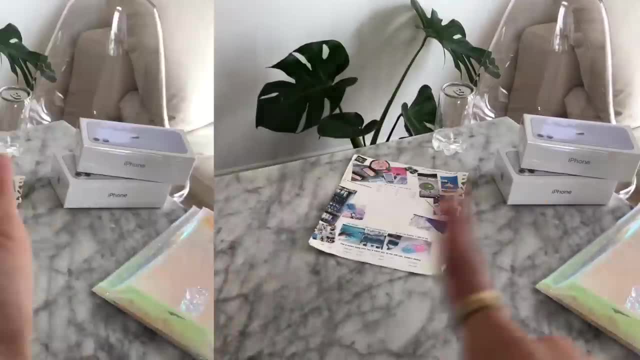 so I can show you guys a studio tour soon, because it's really cool now. so my slime room is all redone and also I've been working on my water slime bottles that you guys can now buy. The first question I see that I want to talk about is how does the bottle work? 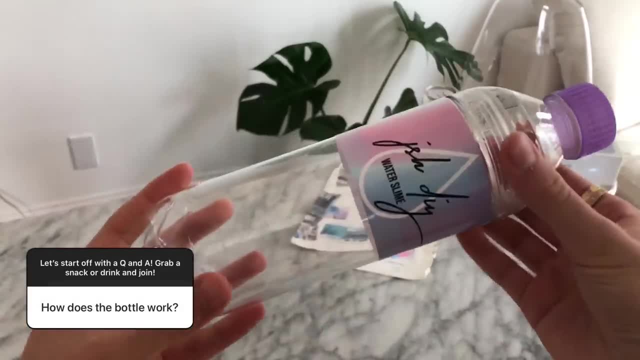 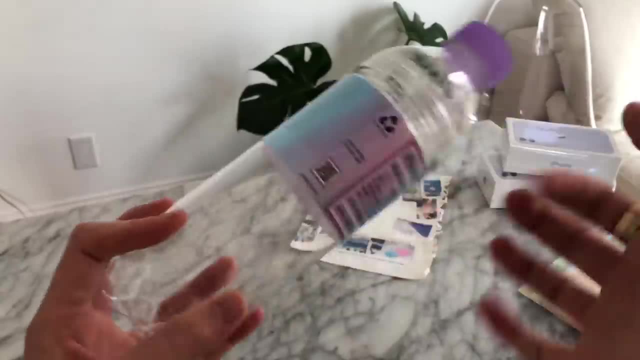 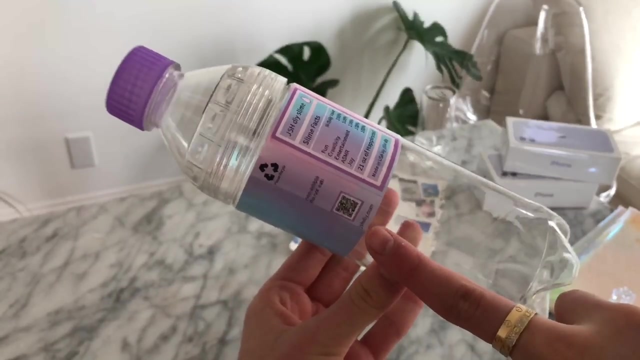 so I have an empty bottle here. So, first off, the storage bottle opens in the middle, which is super cool. Also, the bottle is engineered to actually clear up your slime quickly once you put it back in the bottle to sit. The second thing I'm going to tell you guys about is the magic QR code. 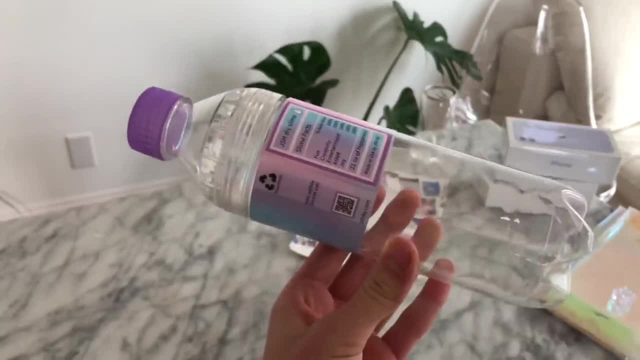 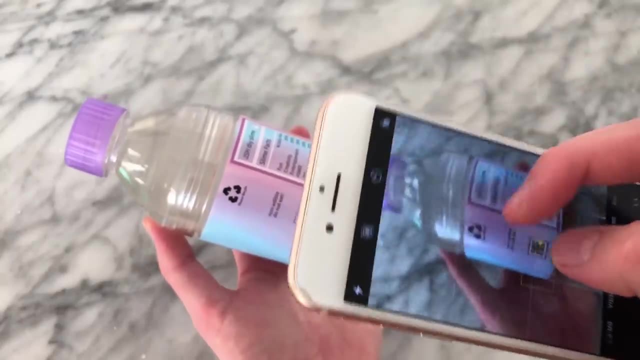 that is on the back of the bottle. I wanted it to be that if you buy a bottle you get endless fun. but the back of every bottle there is this little special box and when you scan it on your camera, it takes you to a magic link. 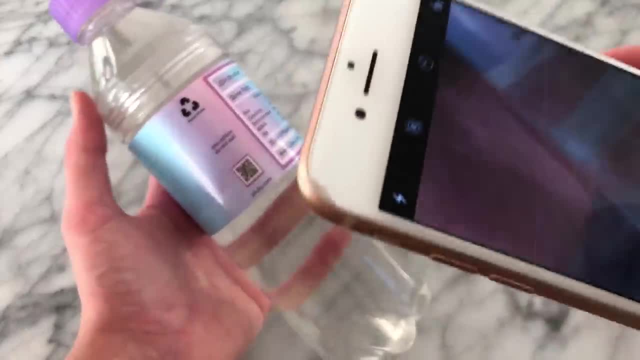 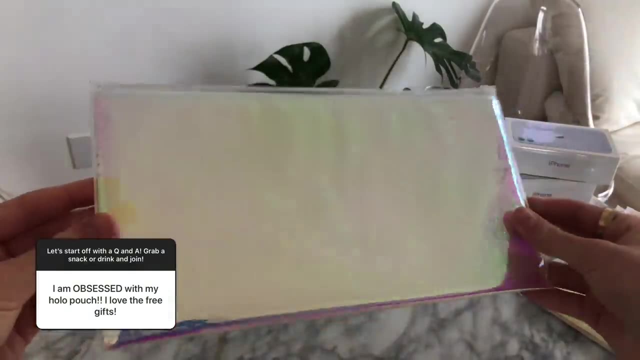 especially for you from me. that is full of surprises. When you scan it, it's like opening a little present. Also, with your order, you will get this free gift, which is our holographic jelly pouch, which is so cute. 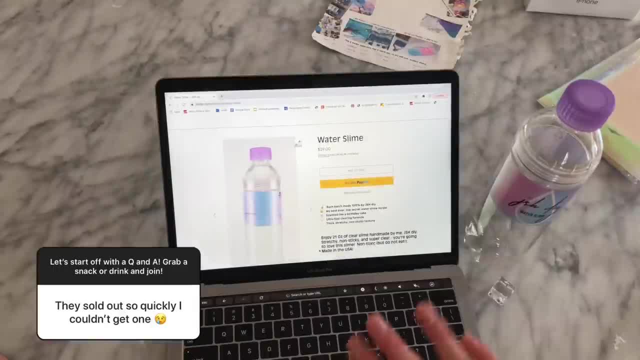 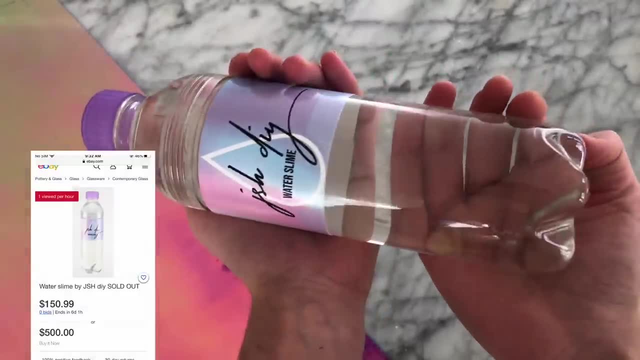 and you can use it for so many things. When I first launched, the bottles all sold out very quickly, but now you guys can all get your hands on a bottle on jshdiycom and you can order yours. Some people were reselling their bottles on eBay. 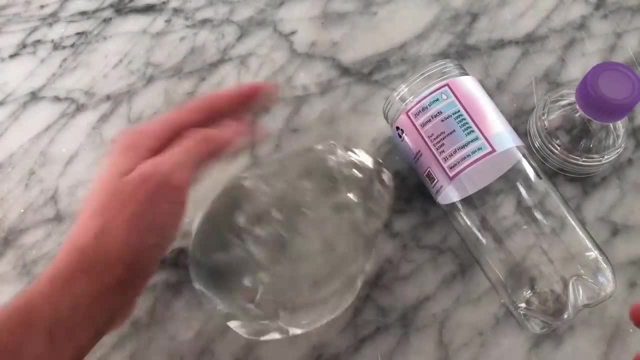 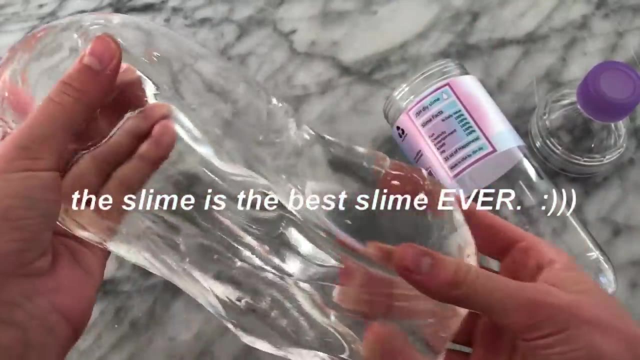 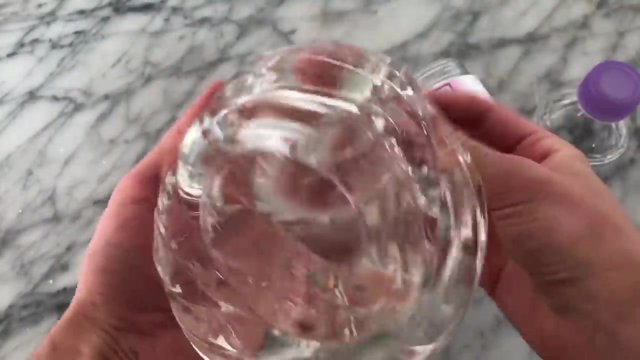 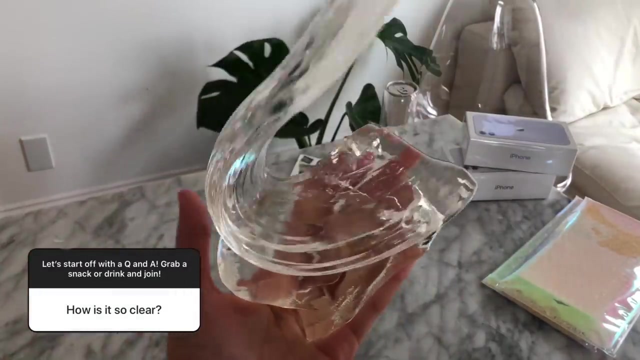 for up to $500, because they were sold out, but you guys can order from my website, jshdiycom. The next thing I want to talk about is the slime itself. So this slime is a crystal clear slime and each bottle is a piece of my perfected water slime formula. 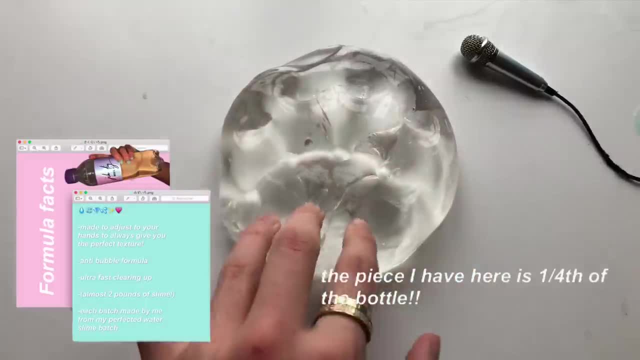 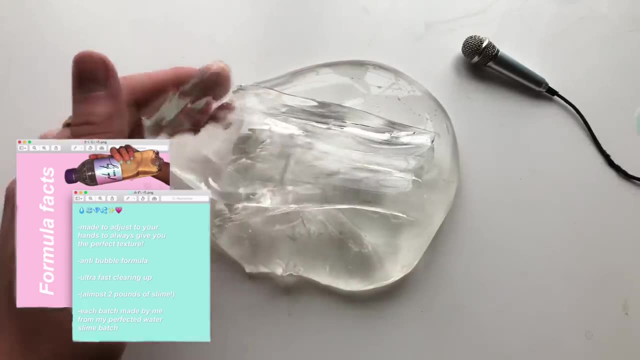 First off, you get about two pounds of water slime. It is a really large batch and it's extremely expensive to make. The clear slime formula is super special because it's anti-bubble, anti-cloud and also is ultra-fast clearing up. 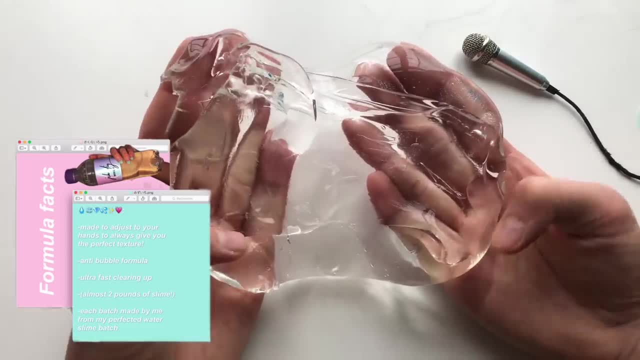 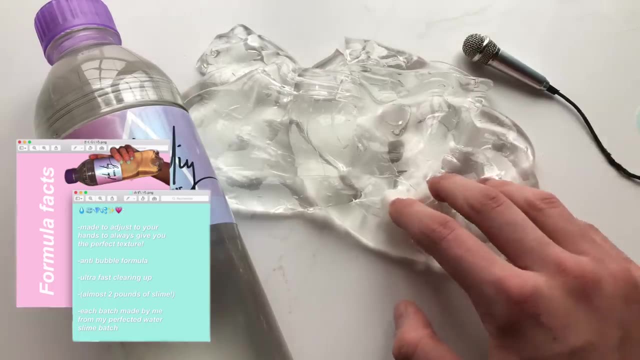 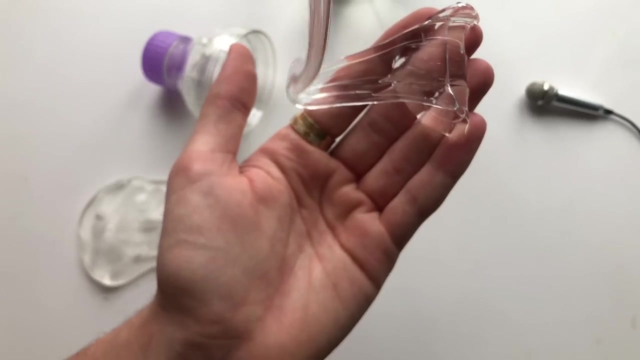 And the slime adjusts to your hands to always give you the perfect texture. and this texture is like nothing you've ever felt before. You just have to feel it, to experience it, because it is incredible. So here is the finished jelly slime. 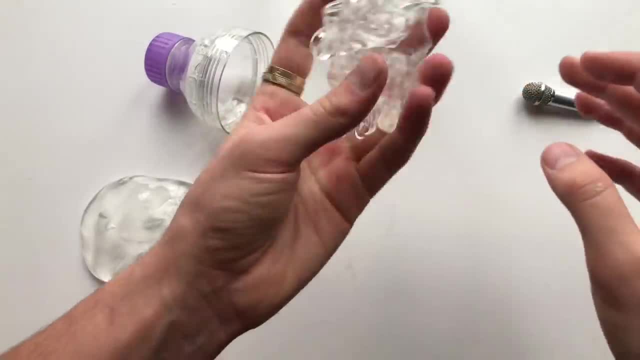 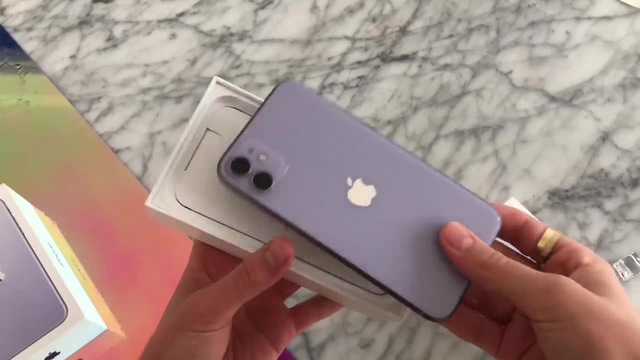 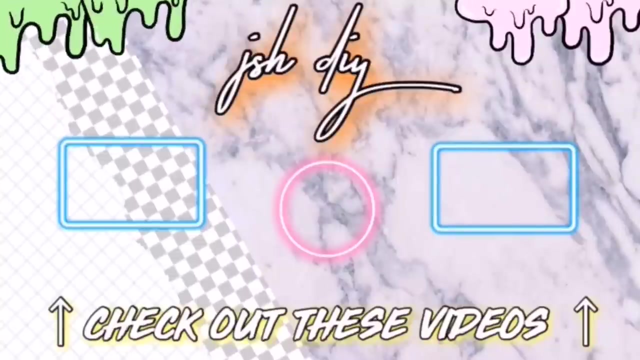 This slime's a اس. In my next video I will be revealing what the golden bottle looks like, but if you get the golden bottle, you will be getting this iPhone also. Thank you guys so much for watching this video. I hope you enjoyed it and I'm so happy to be back.